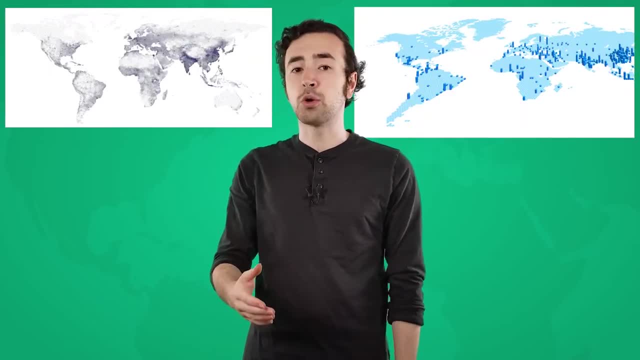 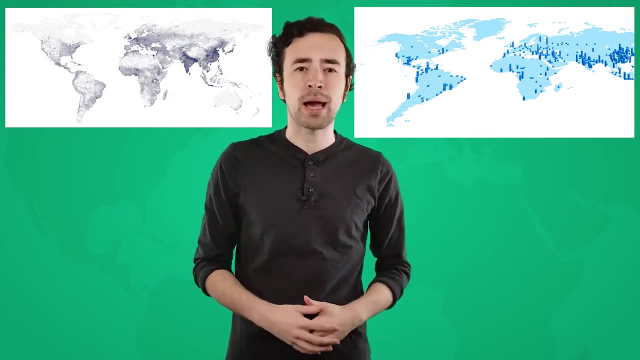 which detail the Earth's features. Other maps include those which show population density, which is how many people are in a given place or area, or other specialty maps like this one which indicates where the world's largest cities are located. Now, these are cool. 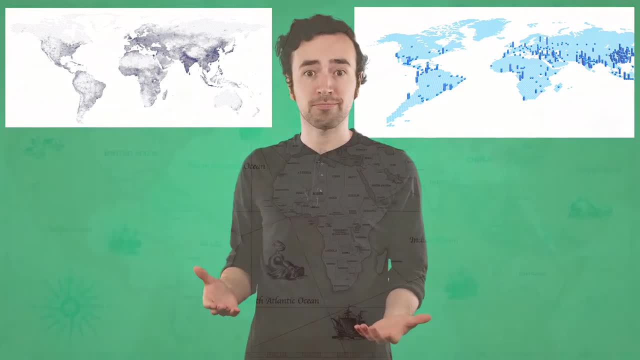 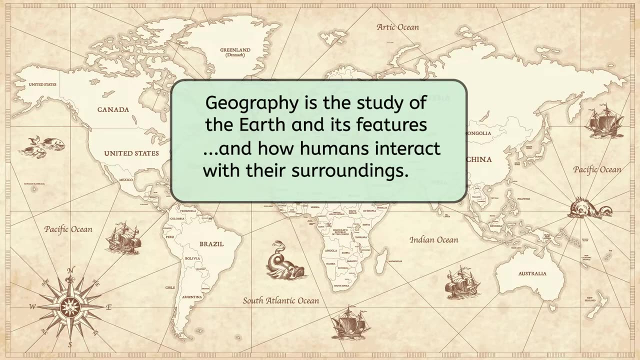 but geography is a lot more than just maps. Geography is the study of the Earth and its features, but it's also the study of how humans interact with their surroundings, which means that geography has been a key factor in the development of all civilizations. 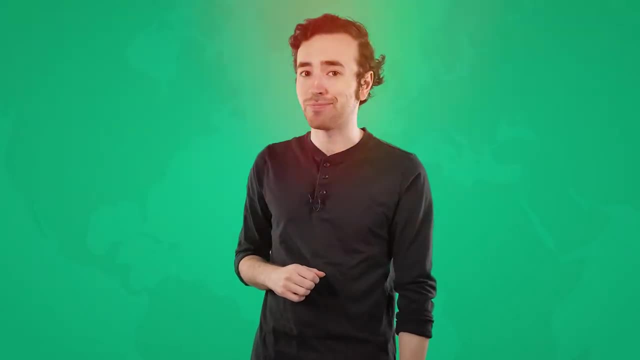 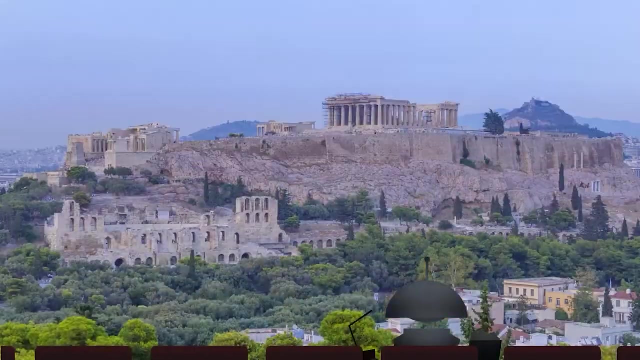 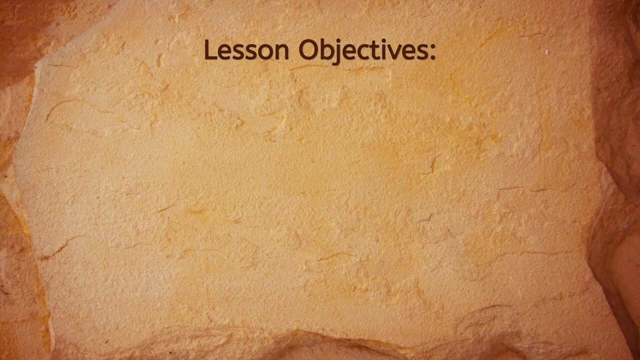 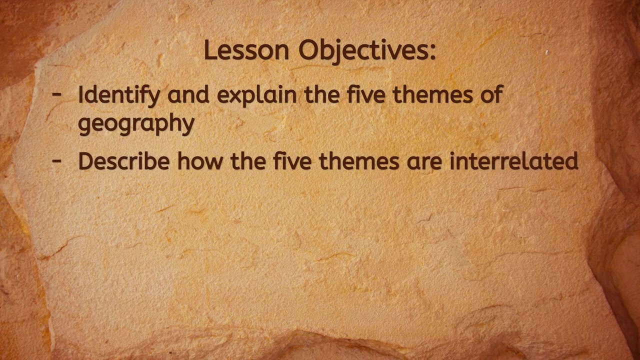 In fact, you might say it's been the foundation. Our objectives today are to identify and explain the five themes of geography, describe how the five themes are interrelated and affect the world around us, and apply the five themes to the study of geography. 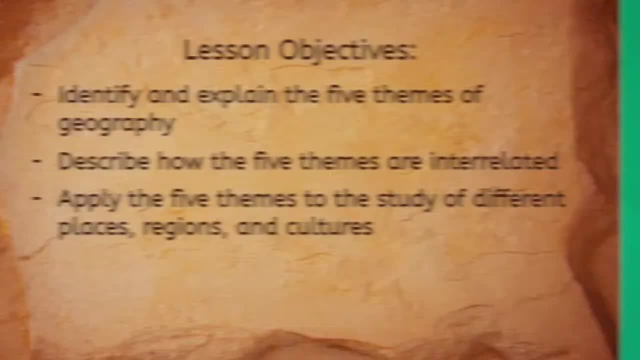 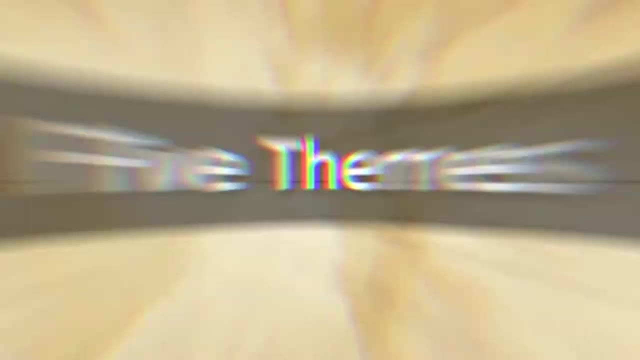 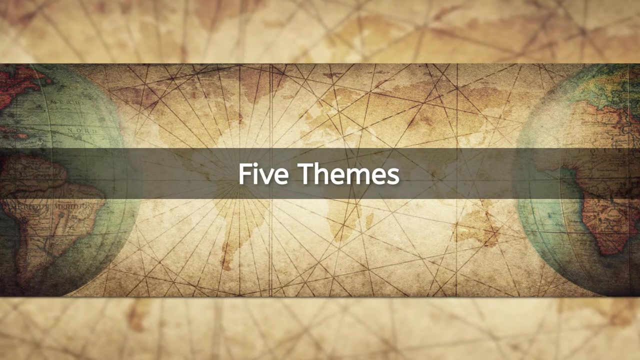 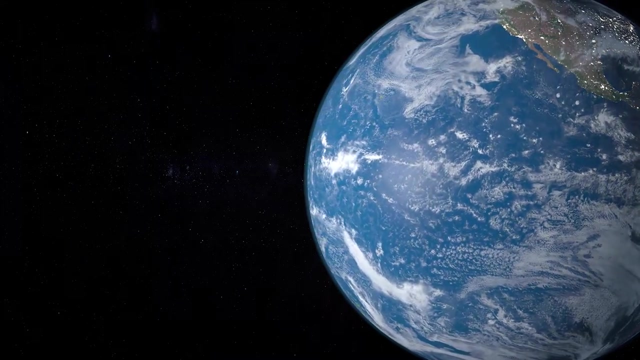 Study of different places, regions and cultures. Ready to tie history and geography together, Let's go. historians, You may already know that 70% of the Earth is covered by water, But most of that is salt water and thus not drinkable. Early civilizations developed near sources. 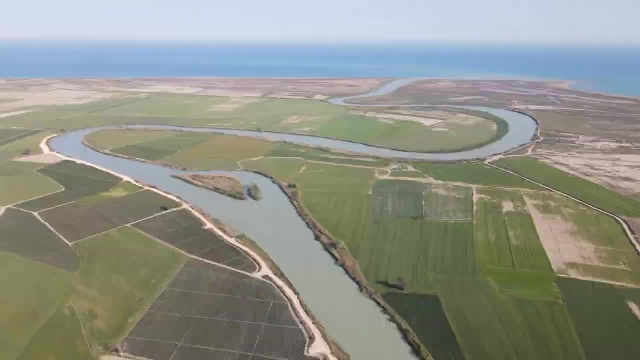 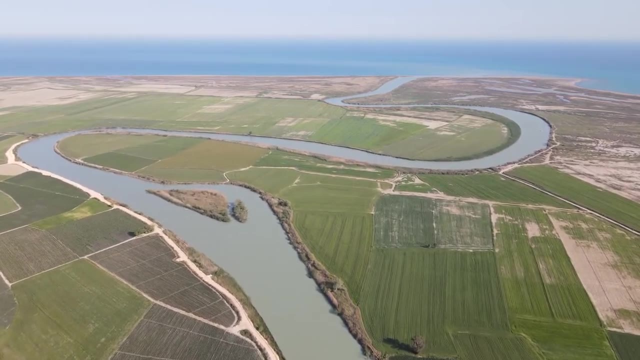 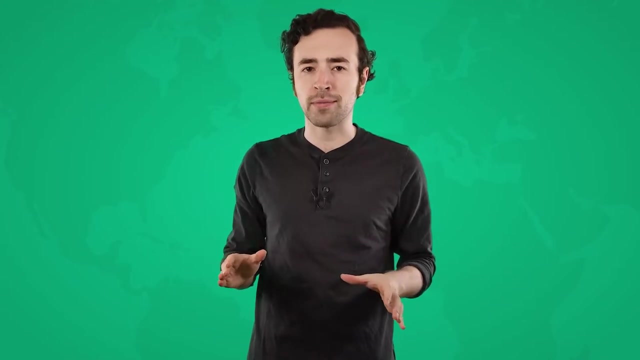 fresh water, which is essential for humans. They needed it to irrigate crops and water animals, to act as a source of transportation and, most importantly, to drink. As we continue to look at where early civilizations were located, you will find over and over again that a water source is key. In fact, it's so important that 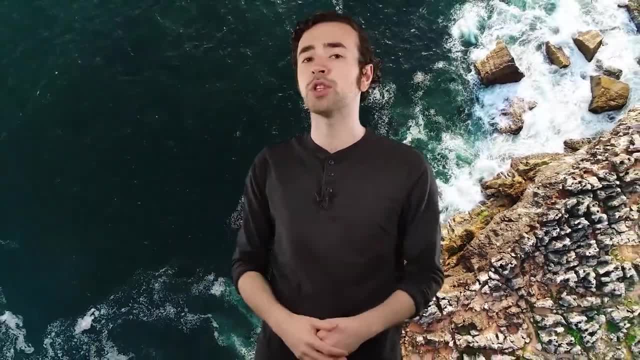 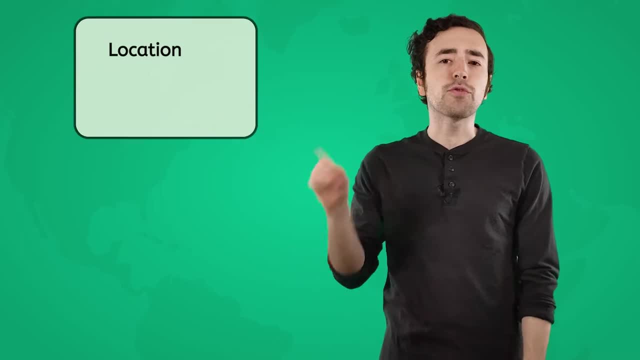 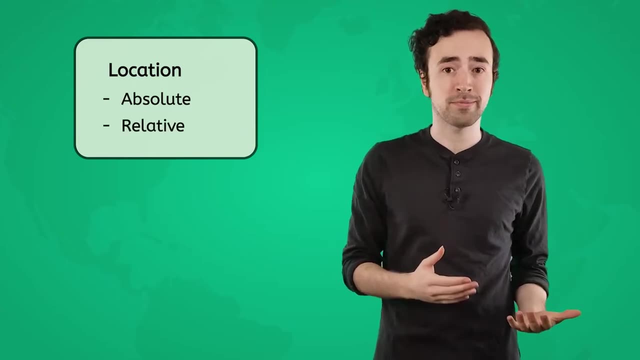 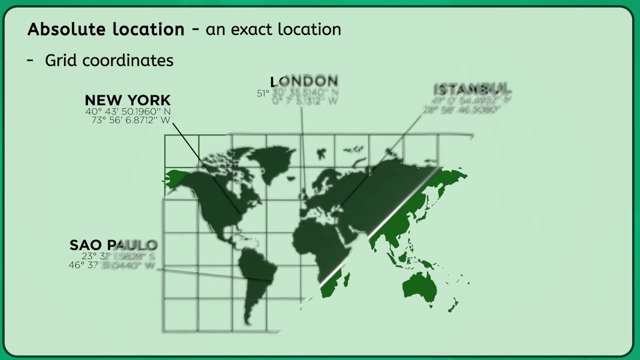 today, as we break down the five themes or parts of geography, we'll be using water as a point of reference for all of them. Our first theme is location. You can have two types of location: absolute or relative. Absolute location means an exact location. To identify absolute location, we use grid coordinates. 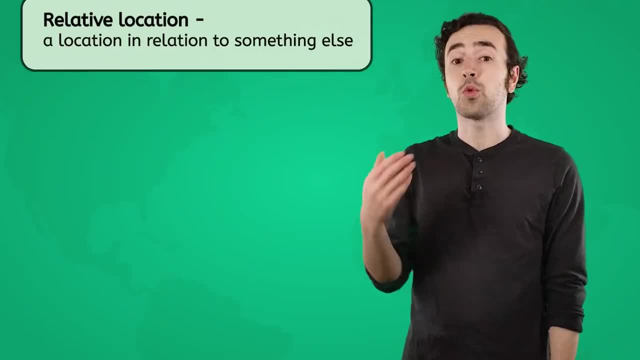 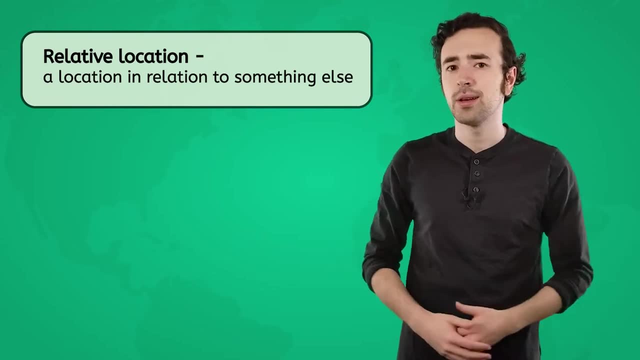 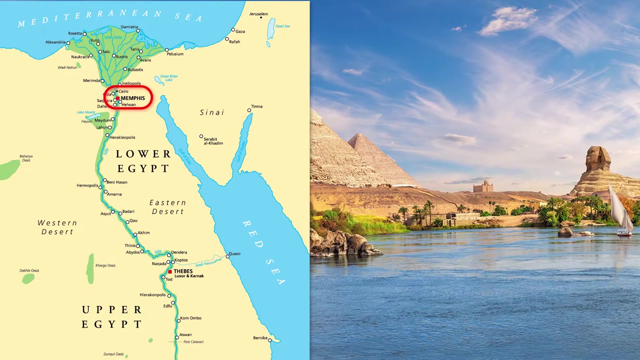 or maybe even an address. Relative location is different. It's a location in relation to something else, like a river or a lake. For example, the ancient city of Memphis was located on the banks of the Nile River, close to the present-day location of Cairo. 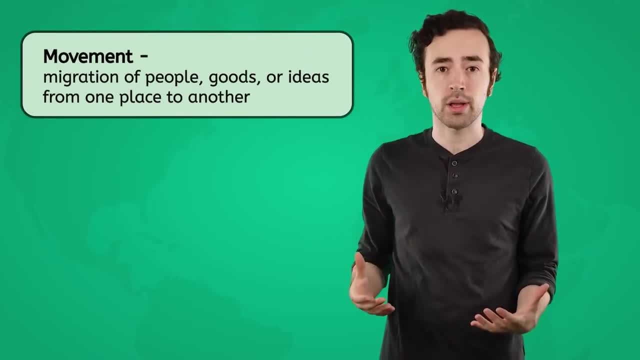 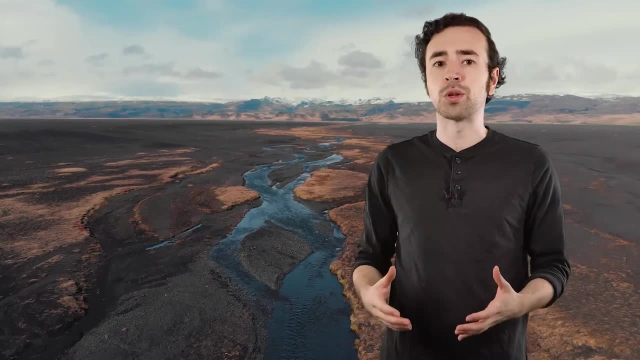 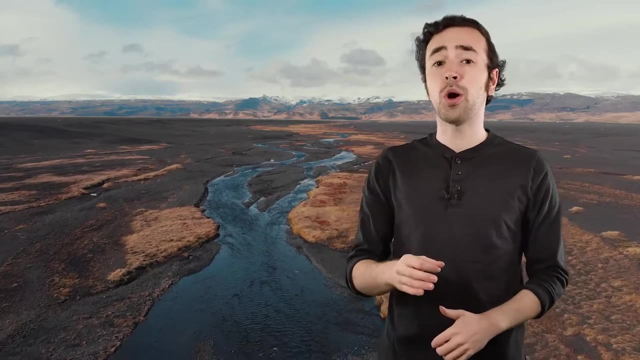 The second theme is movement or migration. It focuses on the movement of people, goods or ideas from one place to another. Finding water was often a reason for migration, because a reliable water source translates to a reliable food source, But it also often served as 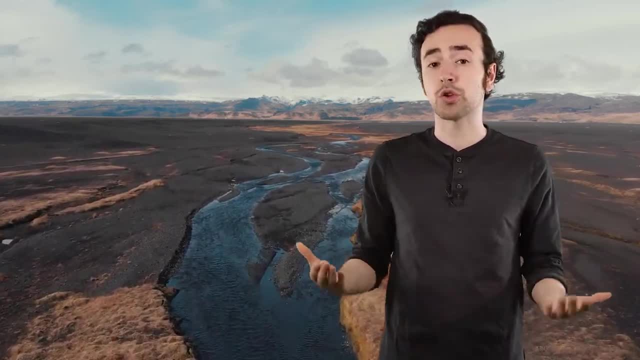 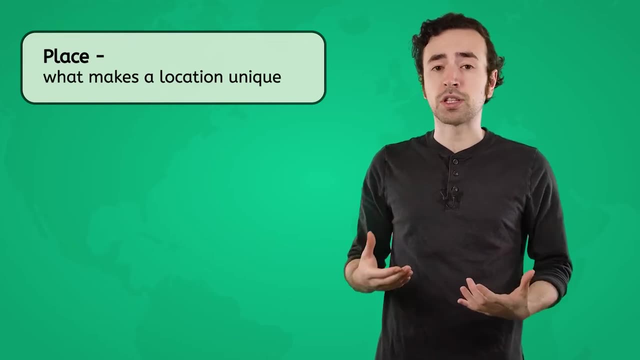 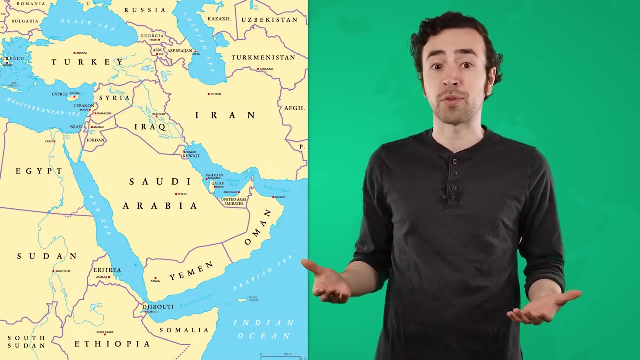 a means of transportation, As people might use a boat to travel. Third, we have place, or what makes a location unique. Those can be either human features, which are man-made, or physical features, which are natural. Of course, some natural features that provide uniqueness to places are bodies of water. 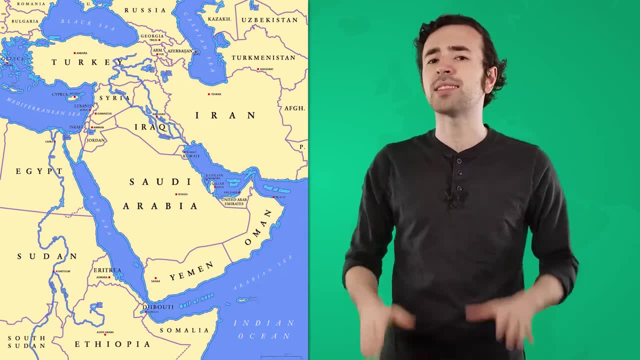 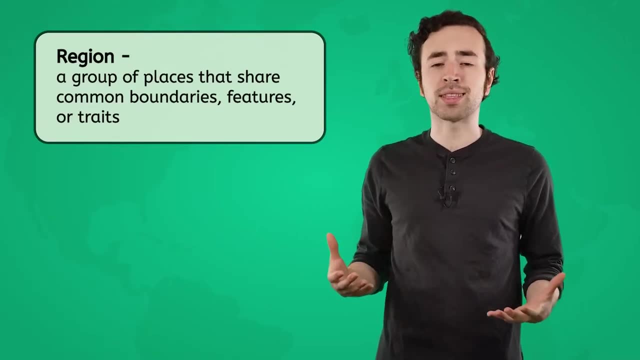 The Middle East, and its access to multiple rivers, seas and oceans is a prime example. The fourth theme of geography is region, which is a group of places that share common boundaries, features or traits. Regions are often determined by a relative location. 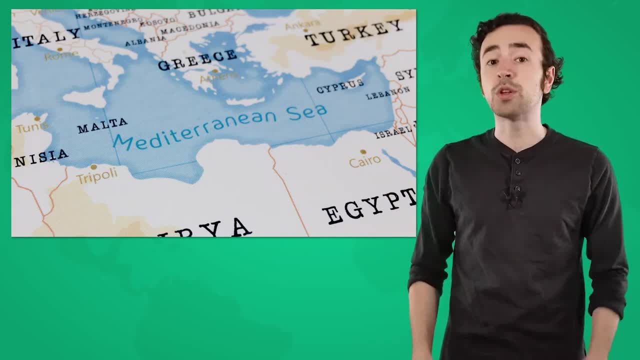 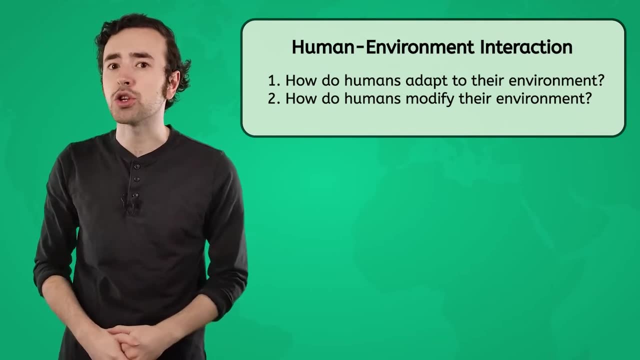 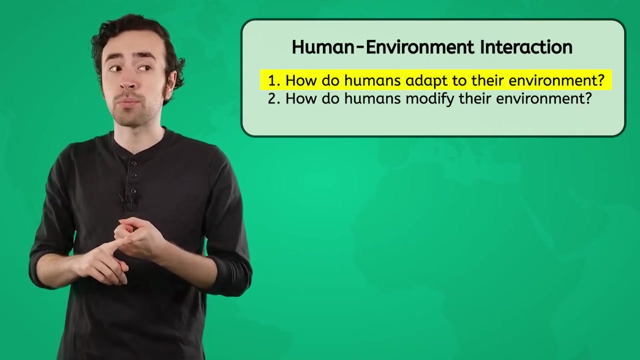 close to a body of water like the Mediterranean Sea, which bordered many ancient civilizations that we'll soon study. And our final theme of geography is human-environment interaction. This theme basically centers on two questions: How do humans adapt or become adjusted to their environment? 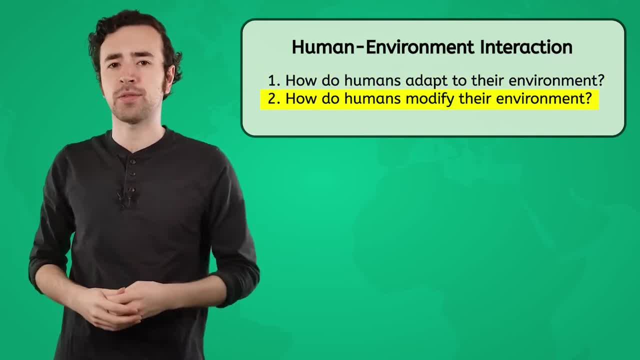 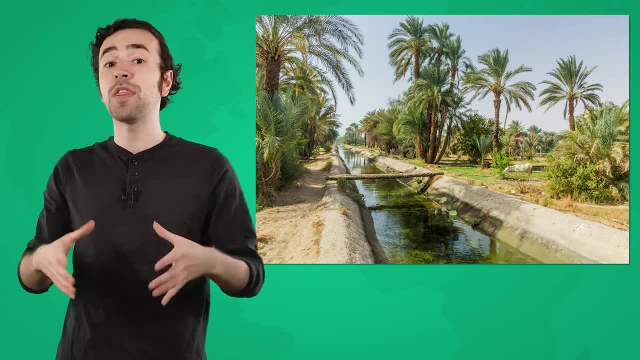 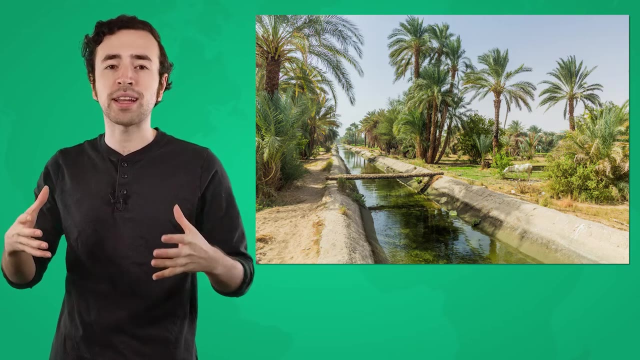 And how do humans modify or change their environment? One interaction that you will notice repeatedly as we investigate the earliest civilizations is how they manipulated water. In particular, pay attention to how they modified the land and used technology to provide a source of water for their food crops. 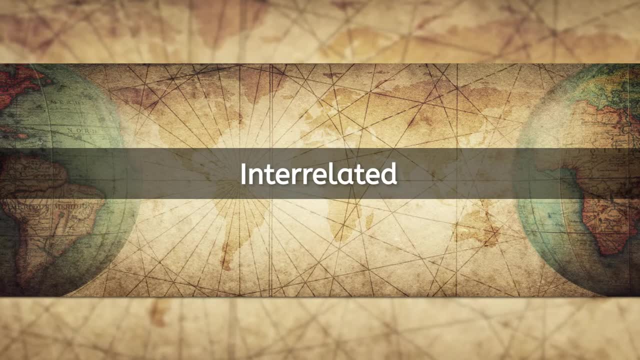 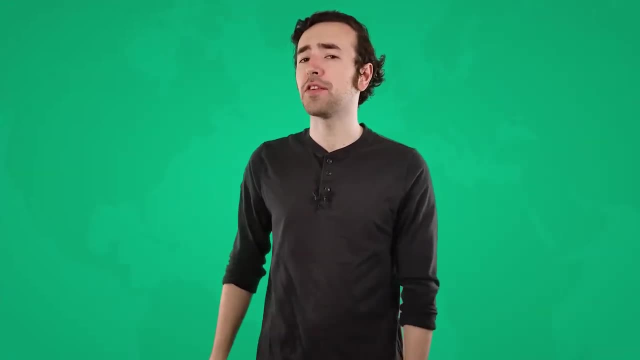 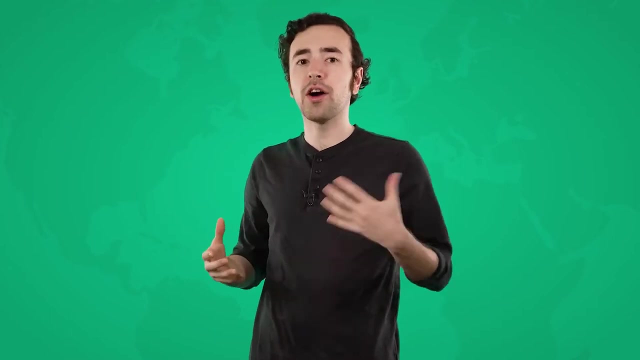 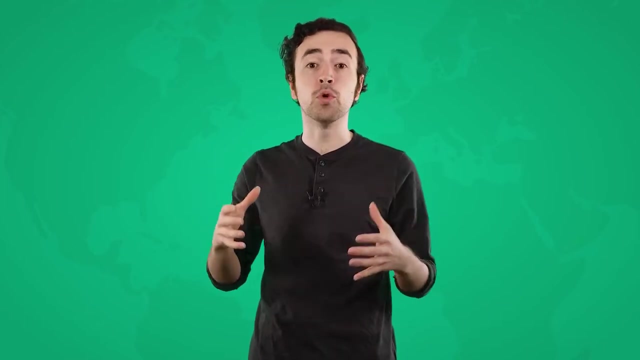 Okay, so we've looked at the five themes individually, but we also have to see them as interrelated, since each one affects the others. For example, the location of a civilization can greatly affect its culture, based on movement to and from the area. 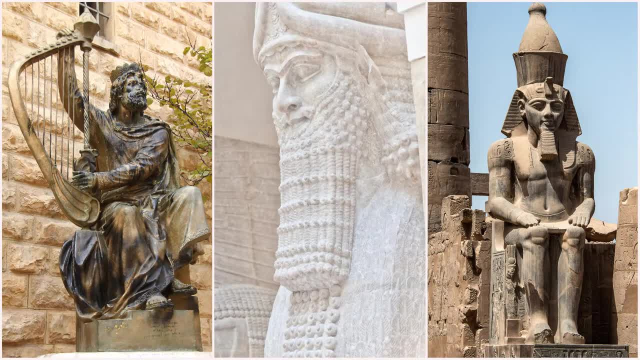 To prove that location and movement are related, watch out for similarities in the political structures of the first civilizations we'll be studying. You will quickly see a common trend that indicates the migration of the ideas of government. In fact, take a moment to predict. 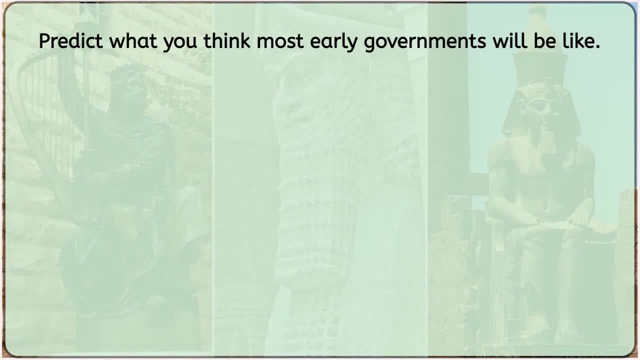 what you think early governments might be like. Do you think most will be a democracy where everyone has an equal vote, An oligarchy where a small group is in charge, Or an authoritarian government where one ruler, like a king, runs things? 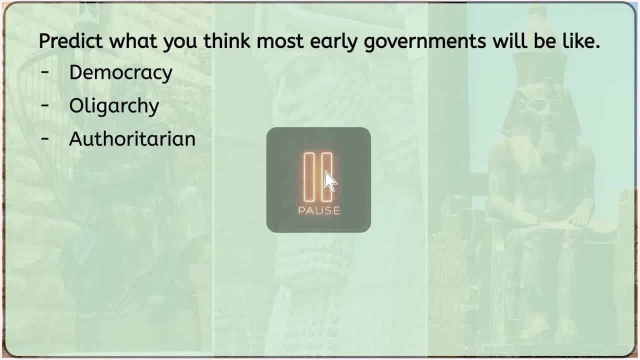 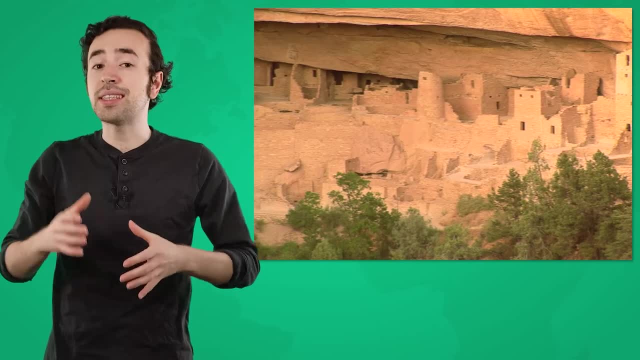 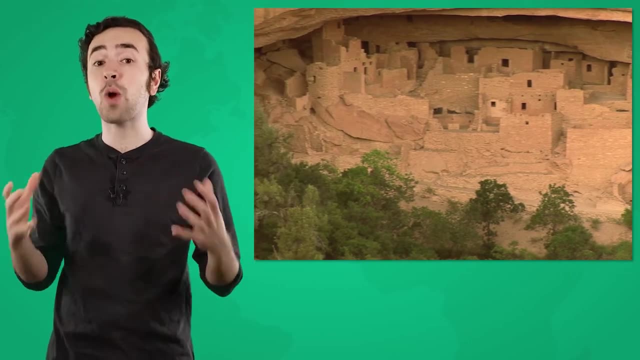 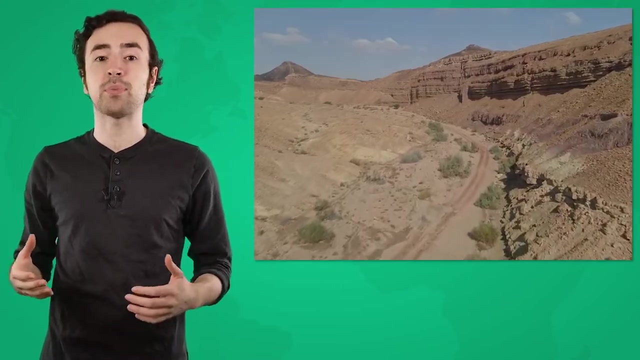 We'll see if you're right soon enough. A second example is the connection between interaction and place. As people adapted to their environment, they used the resources around them to create shelters, like Mesa Verde in Colorado. In Western Asia, the landscape is dry and often desert. 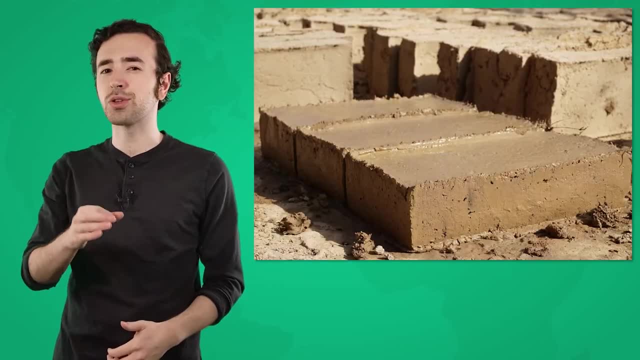 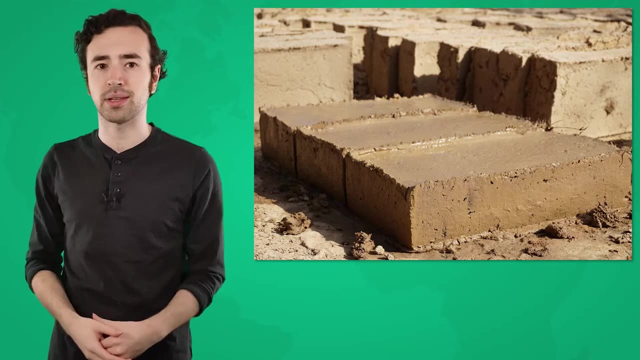 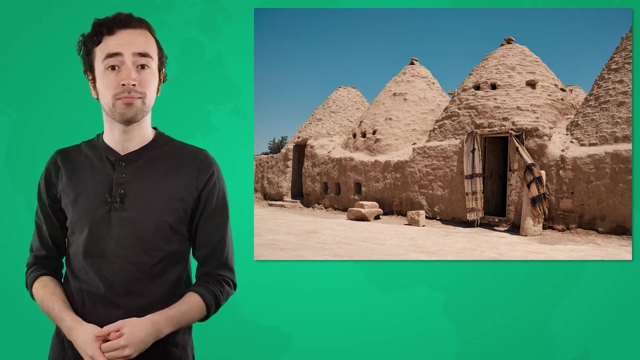 so trees are pretty scarce in that area, So when settlers created shelters, they used water from the nearby rivers to make mud bricks for their homes and other buildings. The homes they constructed made Mesopotamia a unique place, based on the structures that were built there. 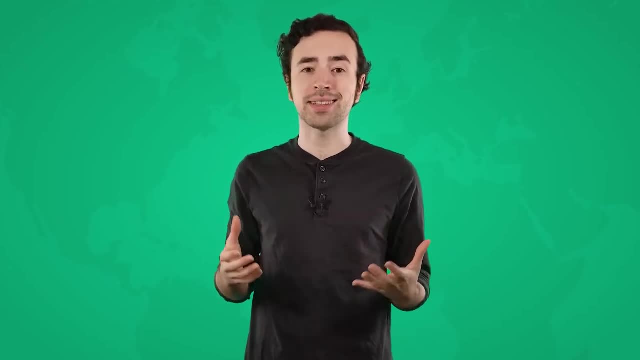 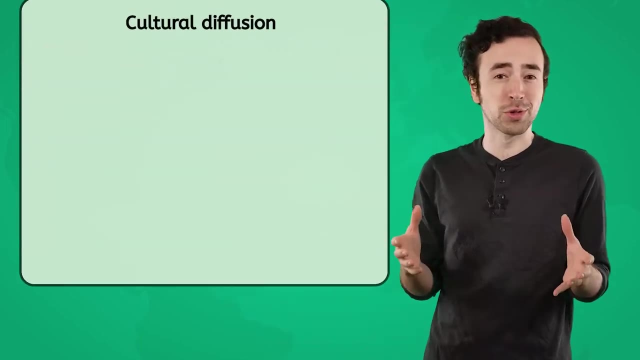 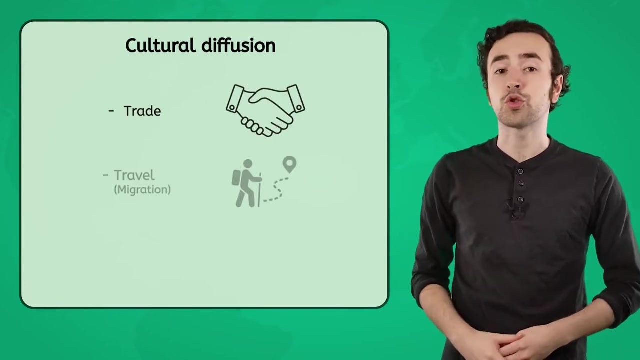 Also be sure to think about the migration of goods, ideas and technology from one location to another and the effects that they had on new cultures. Remember cultural diffusion and the three ways that characteristics are spread from one culture to another: Trade, transportation and war. 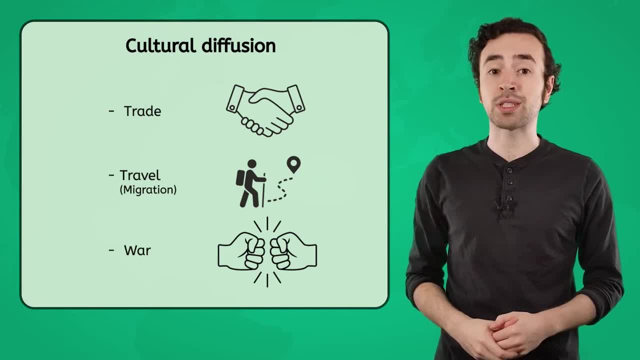 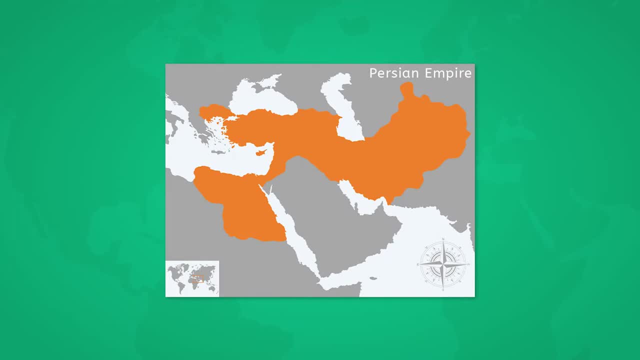 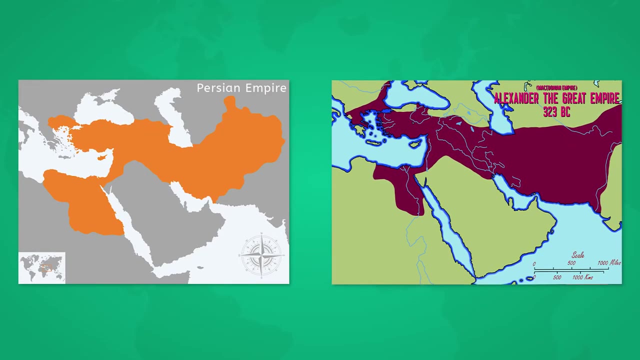 Well, the results of those ideas and technologies being spread around was that new regions evolved over time. For example, look at this map of the Persian Empire. The Persians conquered land and promoted trade across three continents. Now look at this map of Alexander the Great's territory. 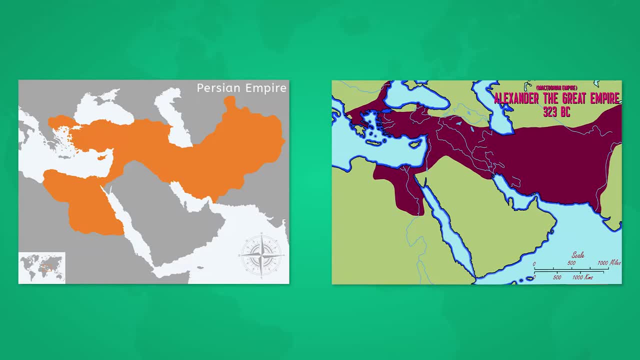 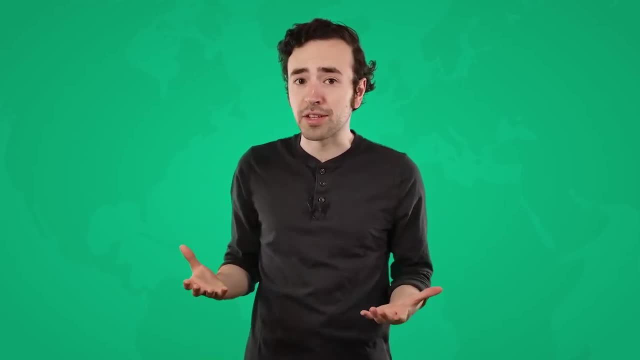 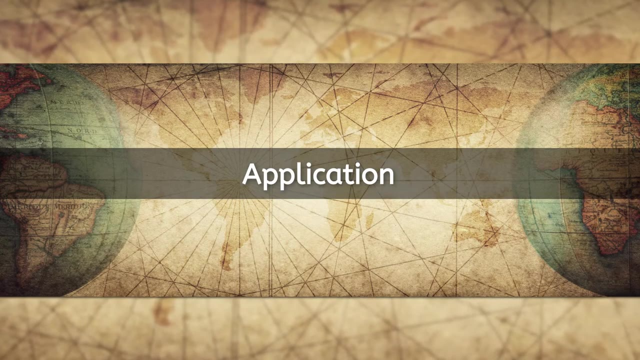 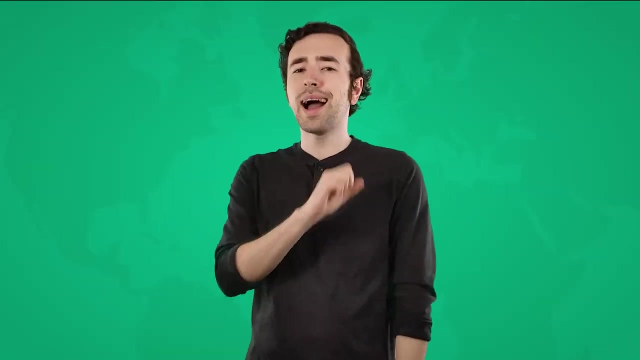 which came later. Much of the same land, but grouped as a different region because of the ruler and the culture instilled. While the five themes are obviously different, they are also dependent on and affect one another. Now let's apply the five themes of geography. 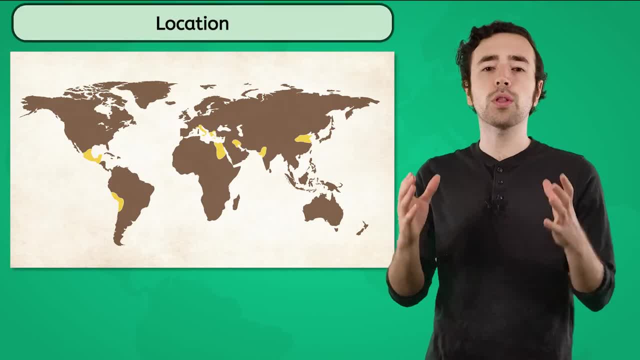 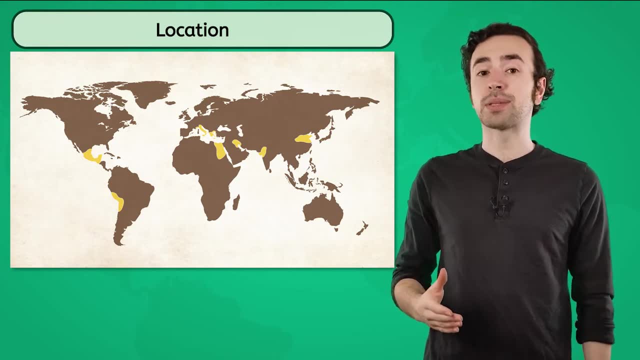 to some of the civilizations we're going to be studying. For location: let's take note of this. For location: let's take note of this. take another peek at our map showing different cultural hearths from around the world. This map helps us to organize their relative locations to some of the Earth's physical features, as well as. 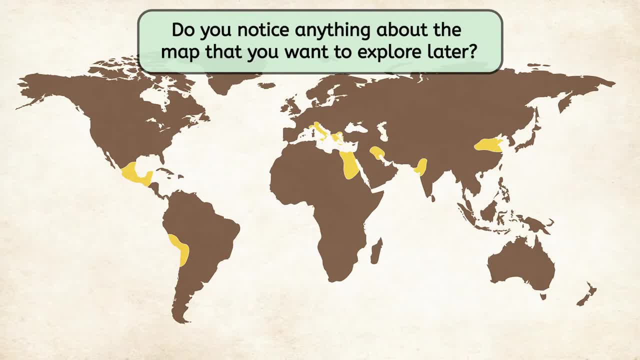 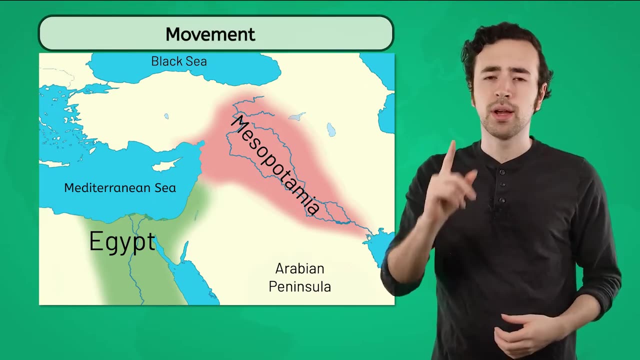 to one another. Do you notice anything about the map that you might want to explore later? Take a moment to write down possible topics for investigation. Let's think about the theme of movement here. In particular, consider the cultural diffusion that took place between the first two ancient civilizations that we'll look at. 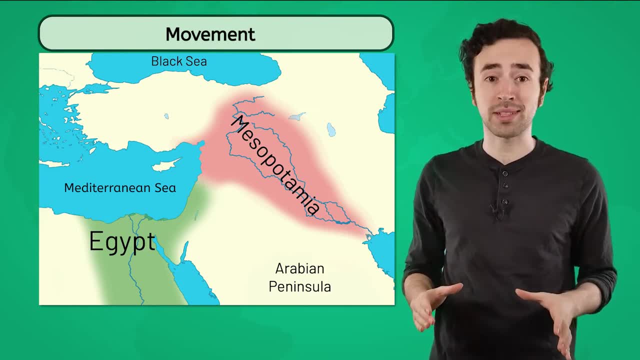 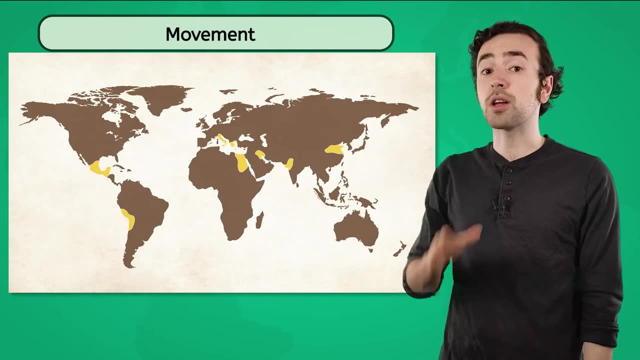 Mesopotamia and Egypt. It's well-documented that city-states in those two regions conducted trade with one another, which makes sense. I mean they're neighbors. But cultural characteristics spread from both Mesopotamia and Egypt, depending on the location of the city-states in those two regions. 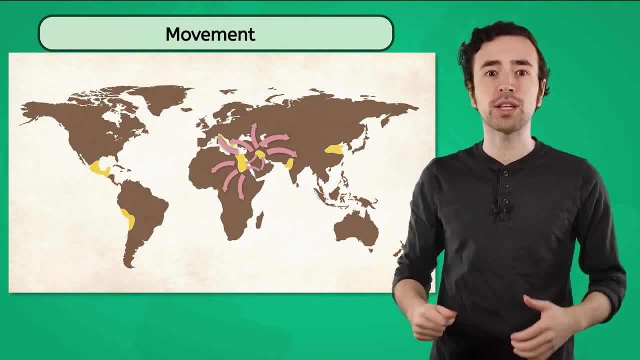 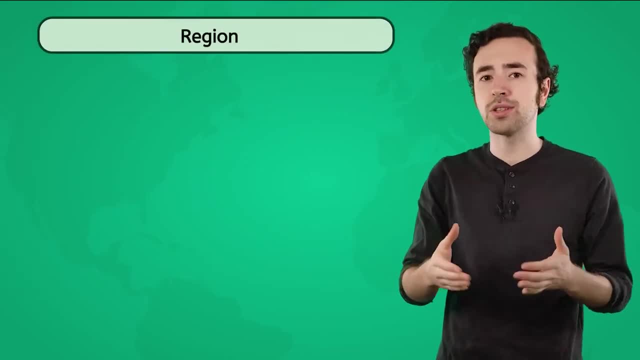 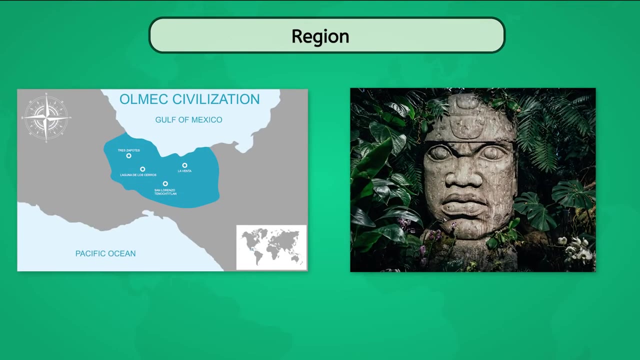 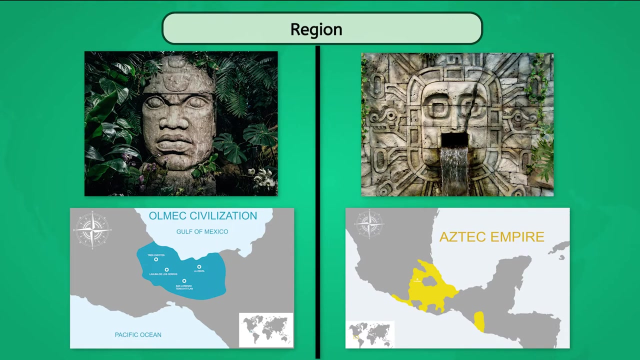 The concept of regions helps explain many similarities found among ancient civilizations and the way they were grouped. For example, the Olmec are considered the mother culture for the Americas, But later civilizations in the region, such as the Aztecs, borrowed and improved upon several Olmec advancements. 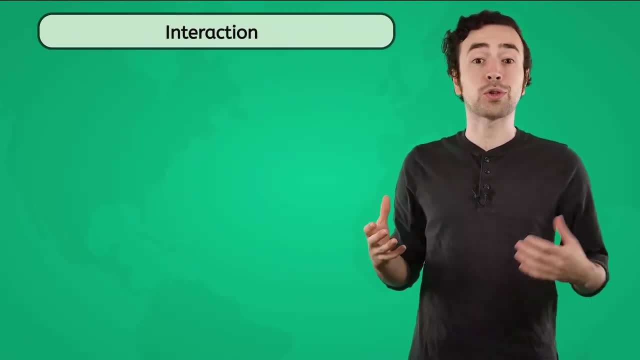 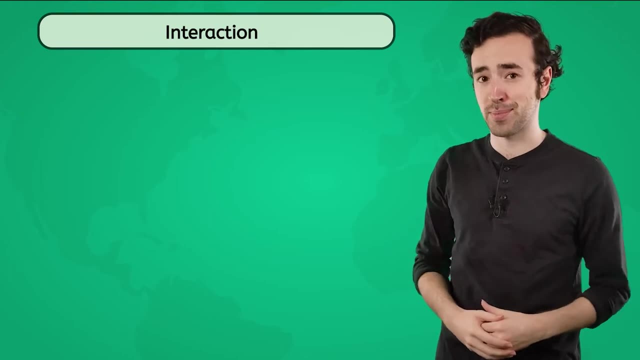 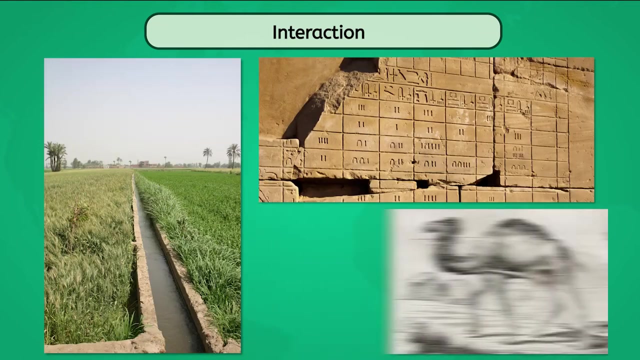 Interaction between humans and their surroundings was the focus of a lot of technology in these early civilizations, which then led to further development. For instance, irrigation methods were created to help with food production, but other developments later helped with planting, cultivating and harvesting crops, Like this Egyptian calendar in the plow. 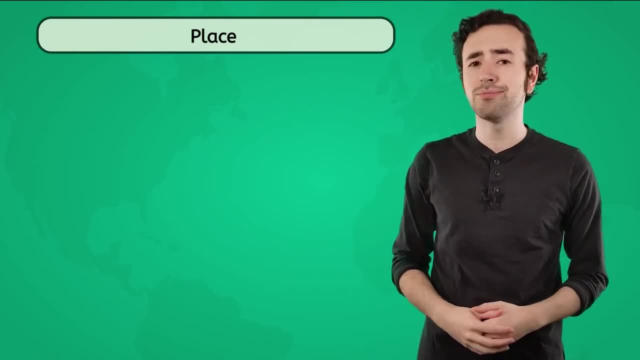 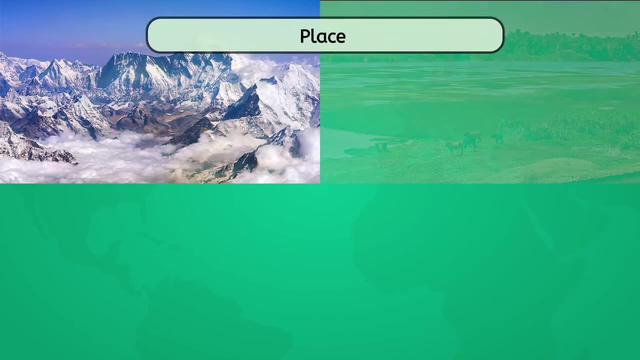 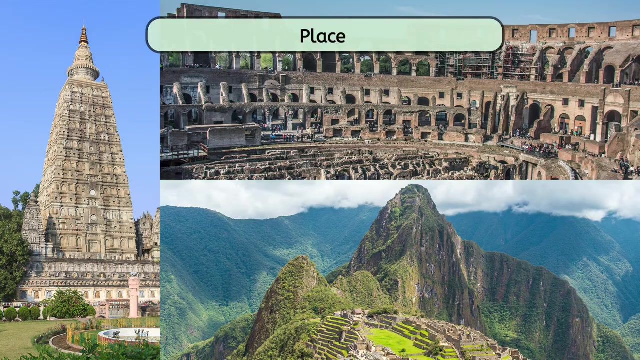 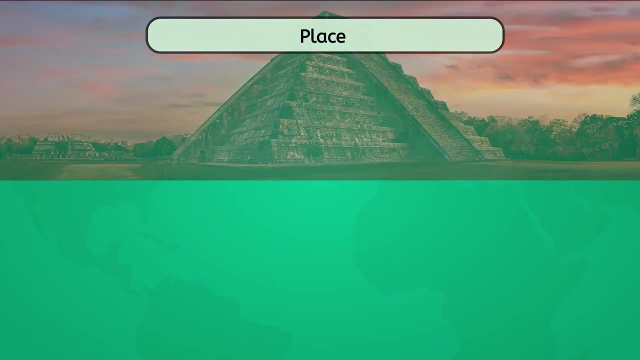 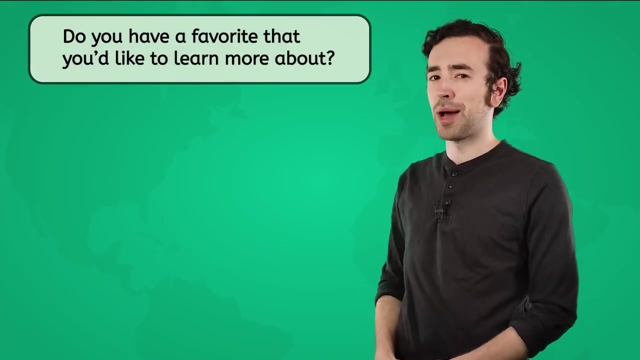 And place, The uniqueness of a location. Well, we're going to see plenty of examples of places that are fascinating and awe-inspiring. Some natural, Others man-made, Many completely one-of-a-kind And others eerily similar. Do you have a favorite that you'd like to learn more about? You might just get your chance. 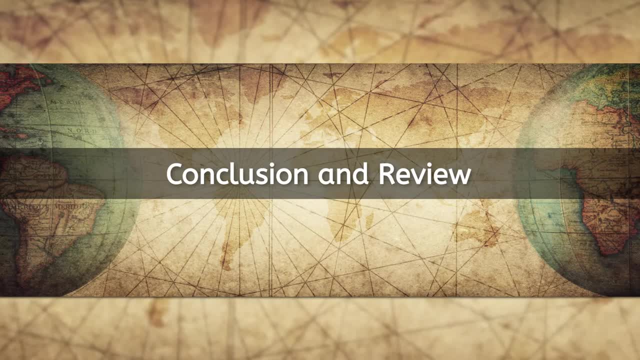 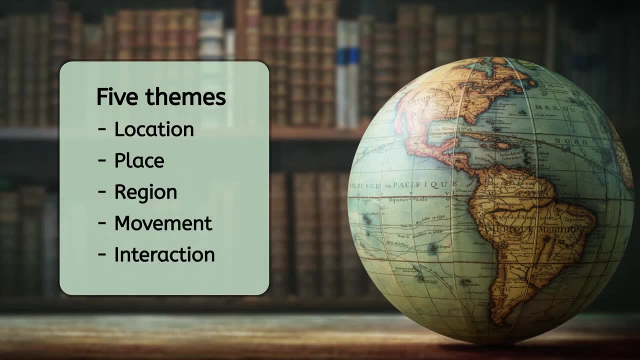 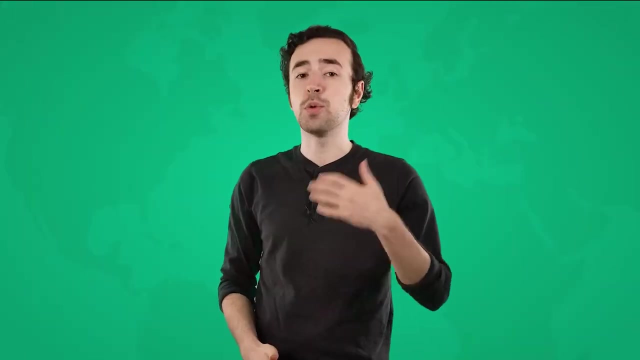 Now that you're familiar with the five themes of geography, it's easier to understand that they are interrelated and essential in the study of ancient history. As we move forward in this course, think about how these apply to each civilization that we encounter.